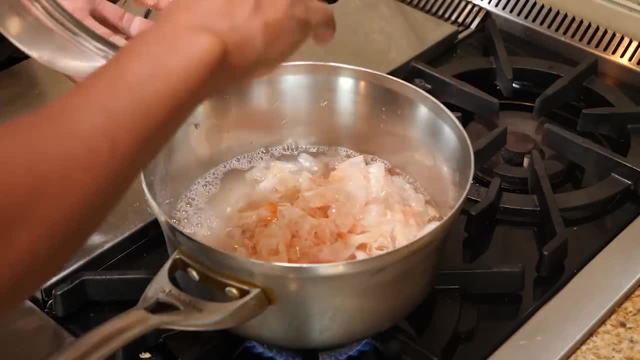 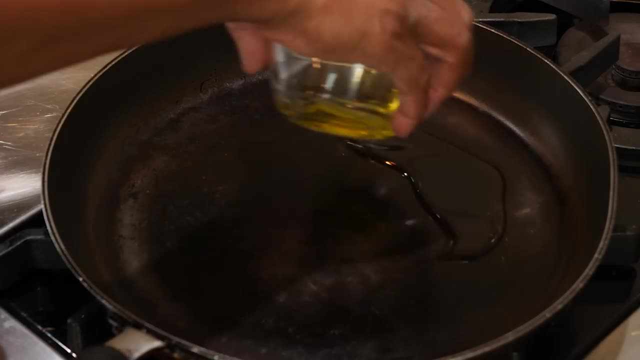 going to keep these shells and we're going to boil them, And this is going to make the most amazing shrimp stock for our gumbo. Okay, so what we're going to do, we're going to take and add a little bit of vegetable oil to our skillet, and I have one pound of sausage. 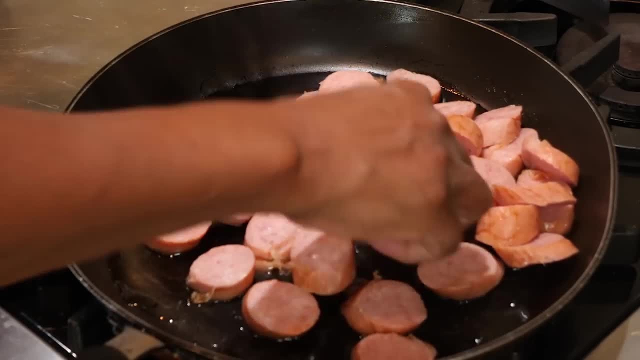 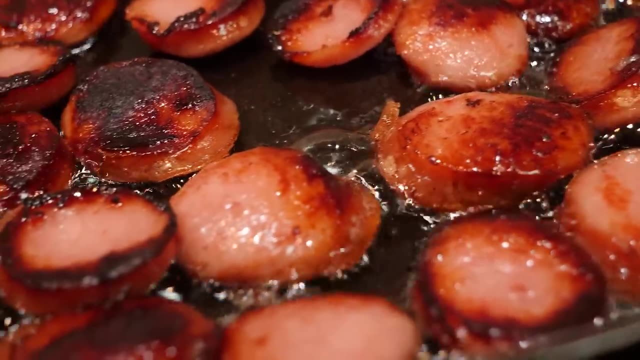 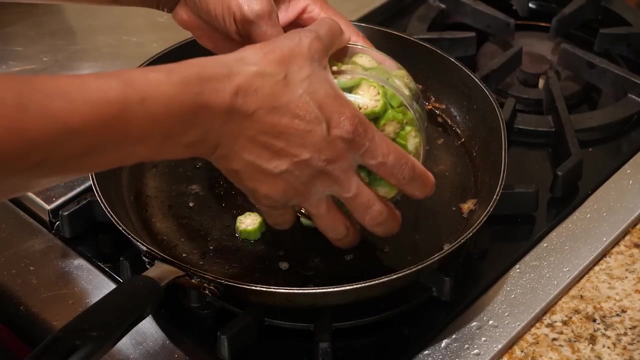 here. Any kind of sausage, andouille sausage, any kind of smoked sausage will work, And we're just going to saute these off, Okay, so the next thing we want to do- we want to. I have two cups of okra, fresh okra. 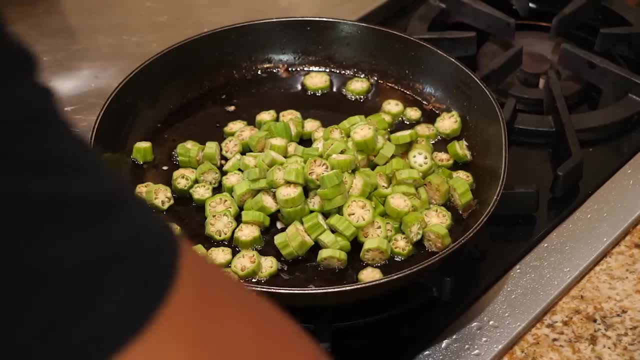 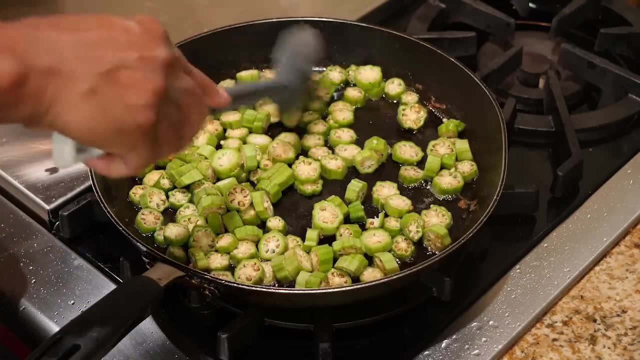 that I took and sliced And we're just going to cook this down until we cook the. We were basically cooking the slime out of the okra because you don't want any slimy gumbo, So we're going to let this cook low and de-slime our okra. 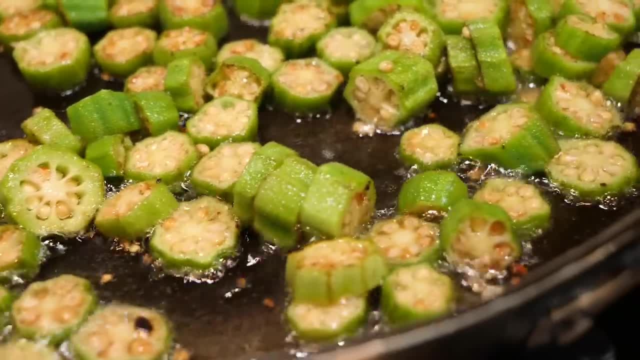 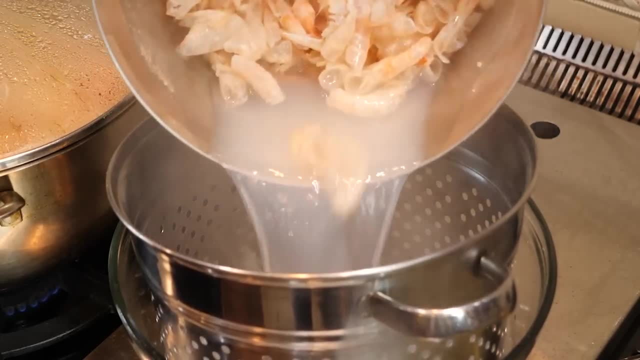 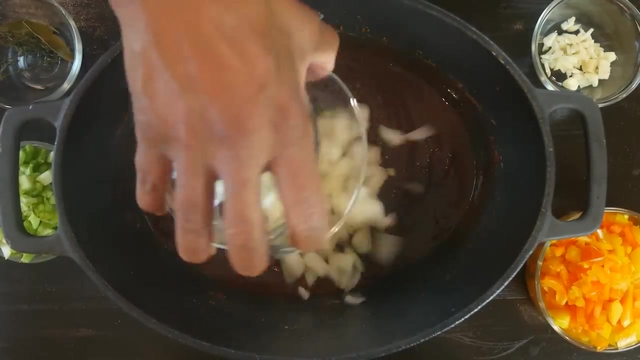 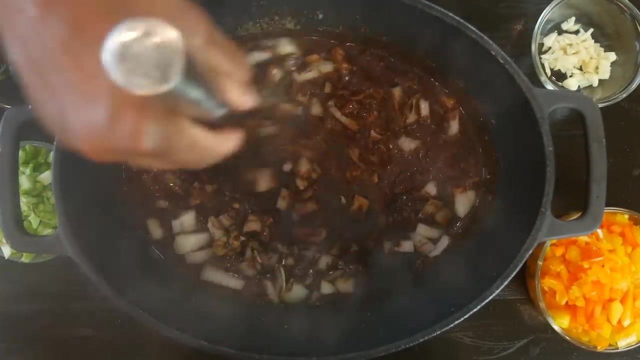 Okay, then we're going to just drain our shrimp shells. This is going to make such an amazing stock. Now that we have our roux, let's go ahead and add in one large onion. That's a large onion. We're going to add in our two bell pepper. You can use green also. 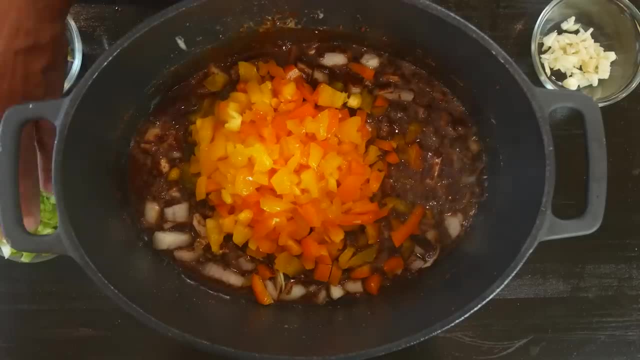 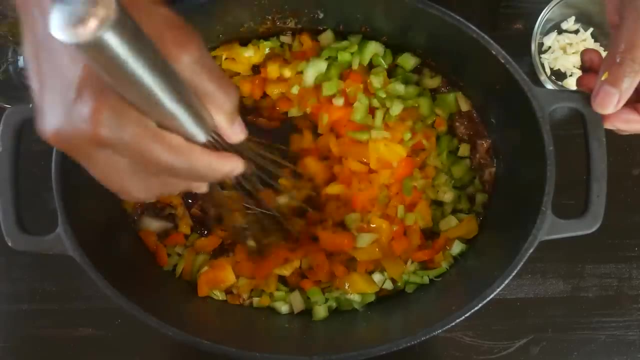 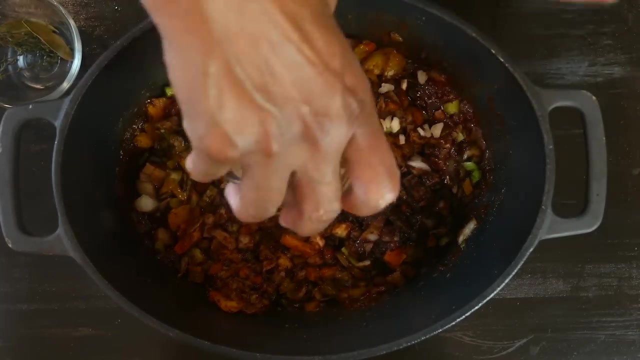 We got orange and yellow. I just like colorfulness. One cup of celery, One cup of celery And we're going to stir all that around. This pot is getting mighty full. Then we're going to take and add in three cloves of garlic. We're going to go ahead and add seafood stock. 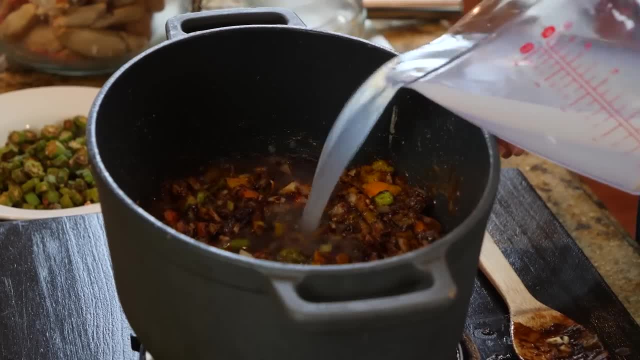 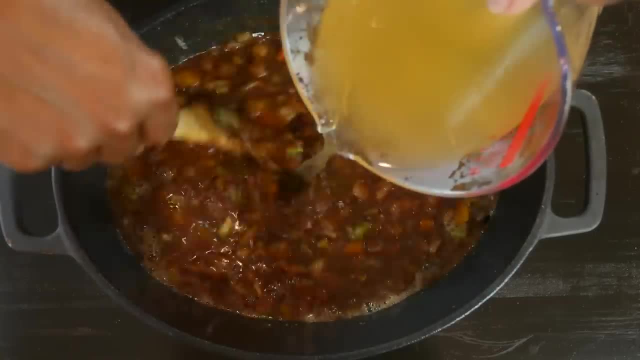 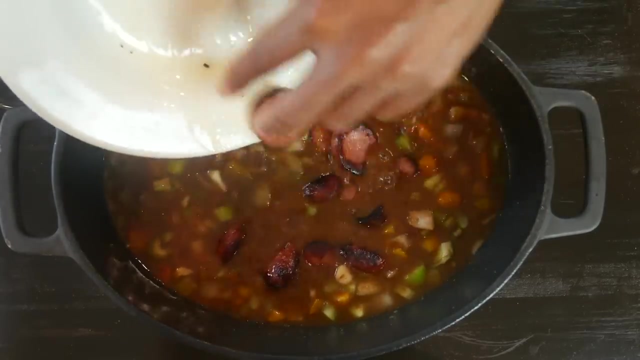 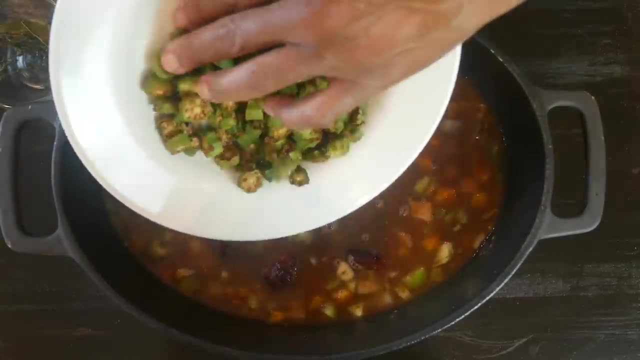 Let's go ahead and add in our chicken stock, Seafood stock and chicken stock. Let's add our sausage that we sautéed off. We're going to add our sausage in there, And we also de-slimed some okra. Let's go ahead and add our okra in there. I'm going to also add two bay leaves. 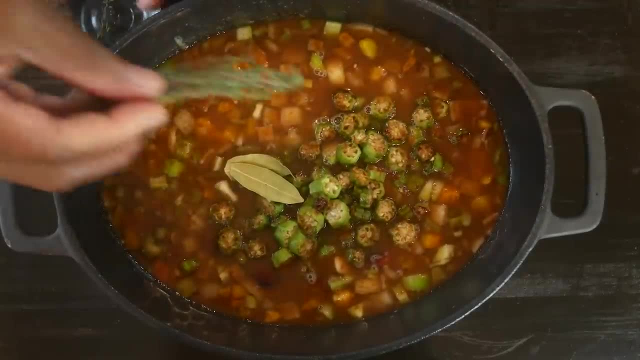 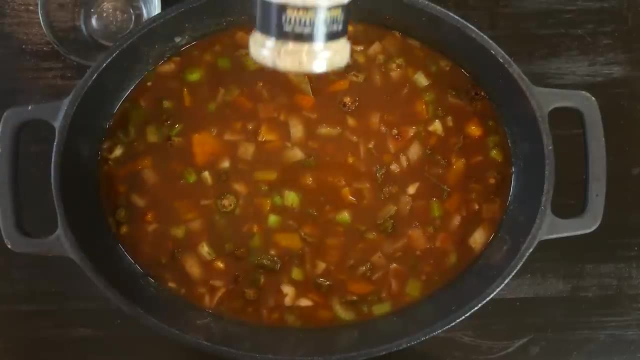 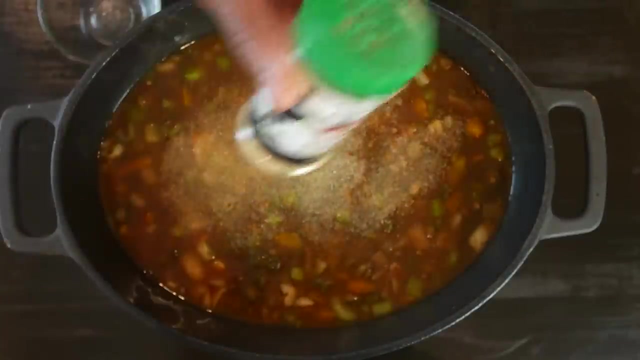 Two bay leaves And I like to add some fresh thyme to mine also, A couple of sprigs of fresh thyme. Now we're going to take this part out. So at this point, guys, we're going to go ahead and add in Chef Carmen's garlic lovers, Because I got you, I promise I got you all. 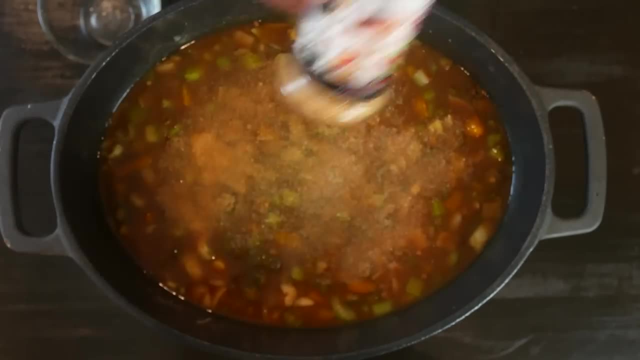 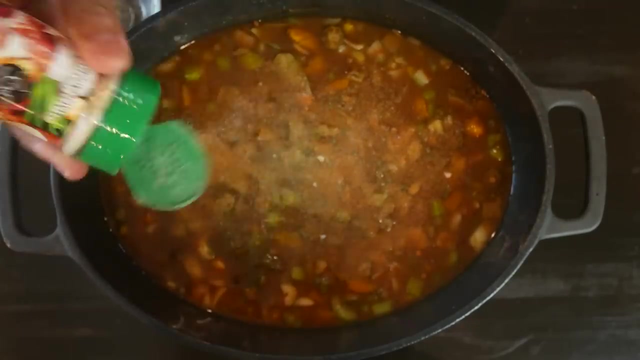 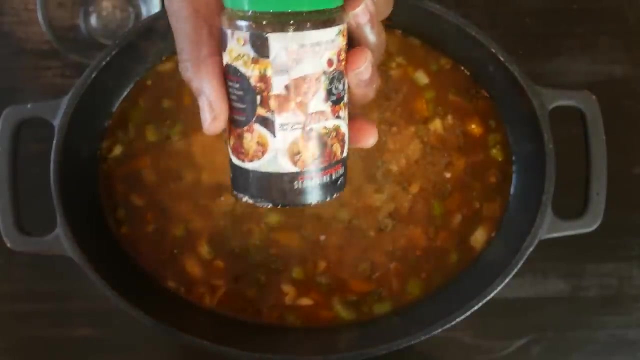 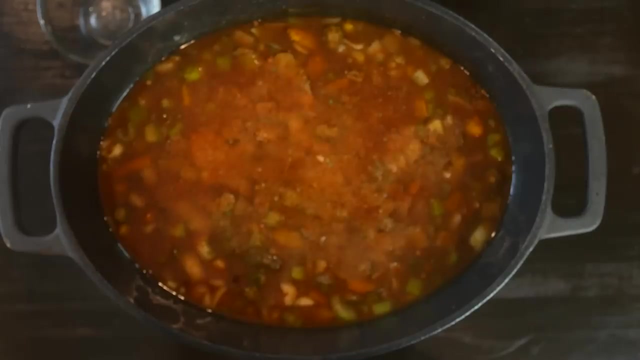 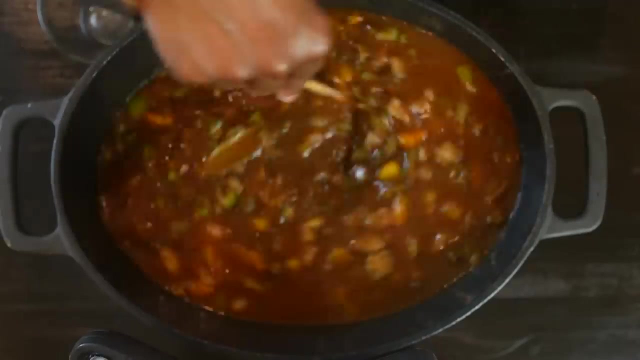 purpose seasoning. I got you onion lovers And we're going to take and add in. I got you Cajun seasoning. Then we're going to take and stir everything up. Simple, easy seafood gumbo. Ain't nothing to it, but to do it, guys, And I got y'all. So at this point, guys, we just want to let. 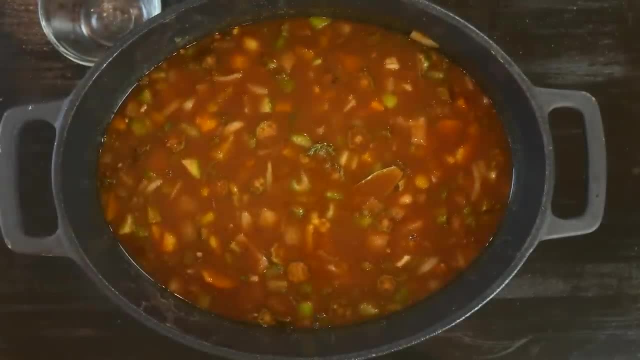 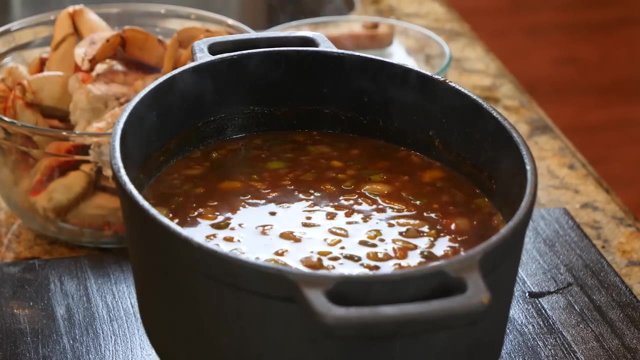 this pot simmer and come to a boil. We're going to let this simmer And come to a boil. We're going to let this simmer for about 45 minutes to an hour. Okay, at this point you want to take and add in your crabs: Crab, crab and more crab. 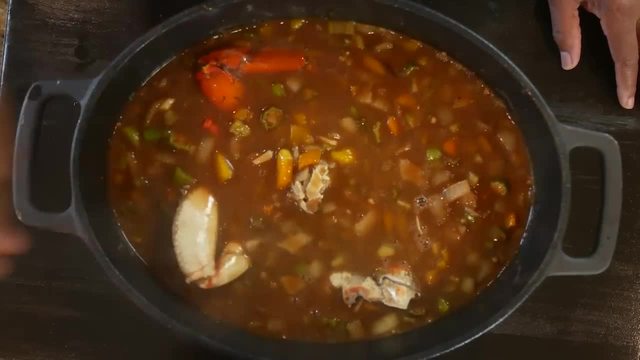 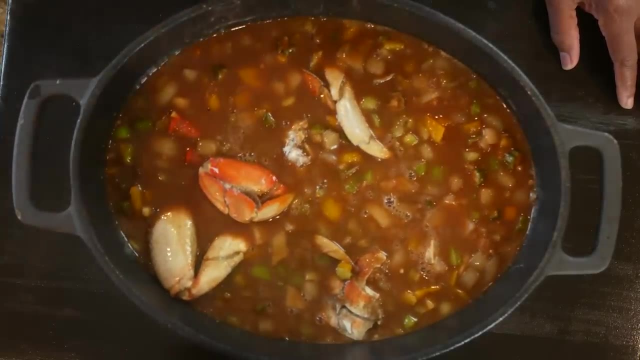 And really your crabs are already cooked, So we're really just warming these up As soon as the crabs get hot. it's done, son, Turn out the lights, the party's over. So we have about three pounds of crab, one pound. 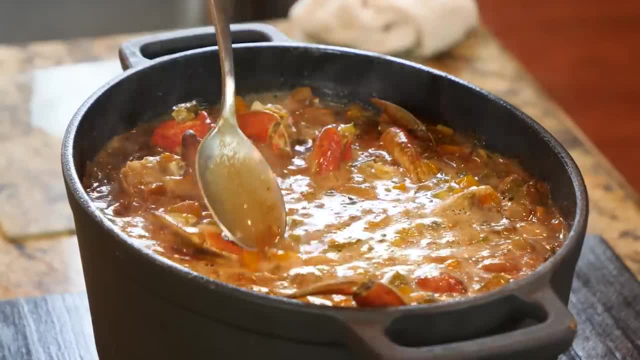 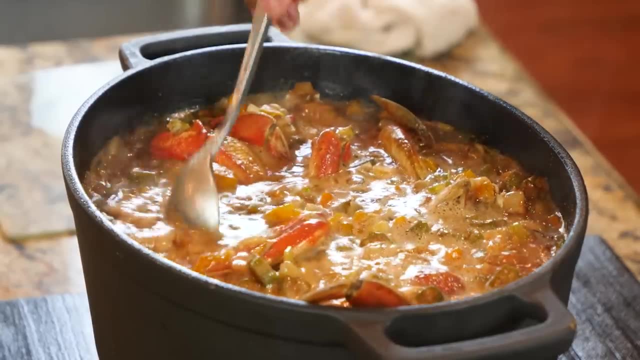 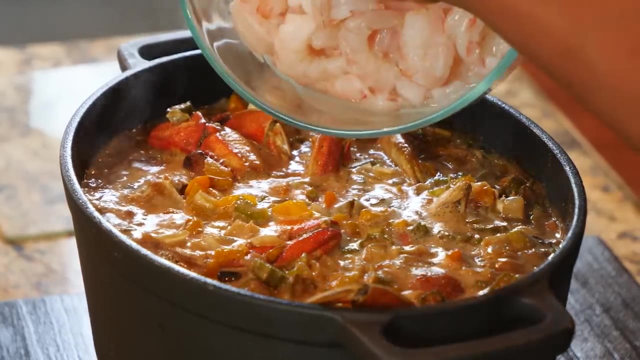 of sausage: one bell pepper, one yellow, one orange, three stalks of celery, two cups of sliced okra, one pound of sausage. So let's go ahead on in and add two pounds of pink shrimp, Gulf shrimp, And in a few minutes it's going to be time to eat, Guys, y'all. 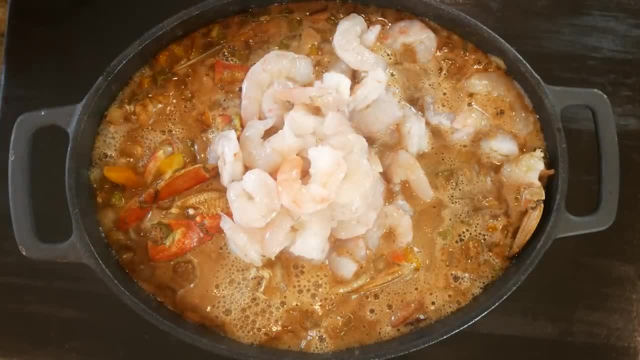 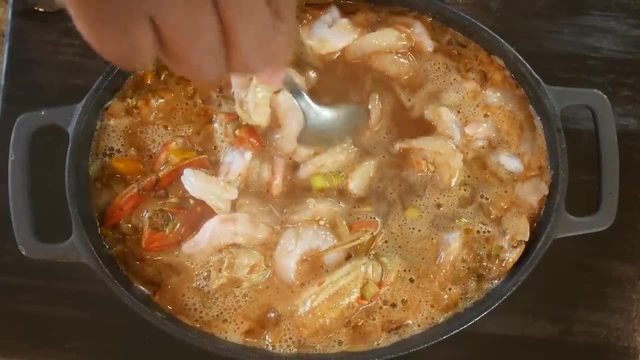 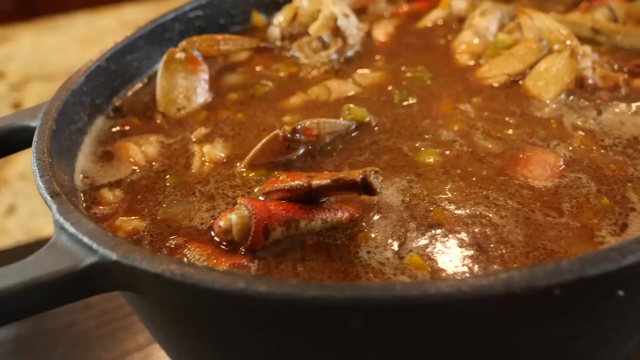 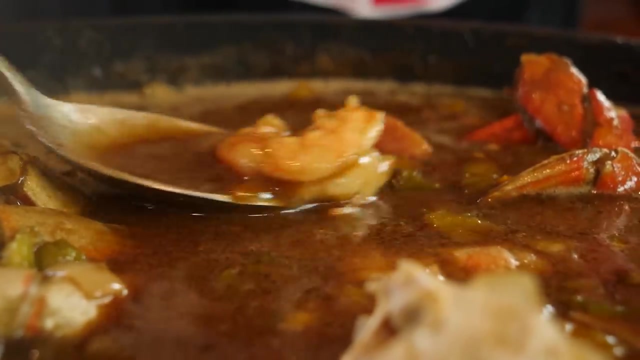 may want a bigger pot for this, And we're going to take and cover it for about five minutes. It's going to be seafood gumbo time, Okay, so let me get in here, guys. I just want to grab one of them. Scram.